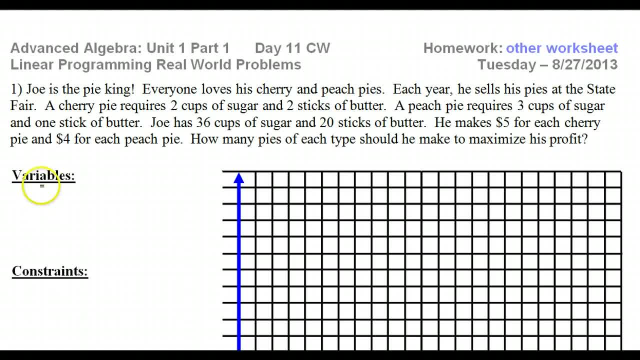 Okay, first thing we do is the variables. All right, this is about pies. I'm not going to read it. How many pies of each type should he make? What are the pies? We've got cherry. we've got peach. 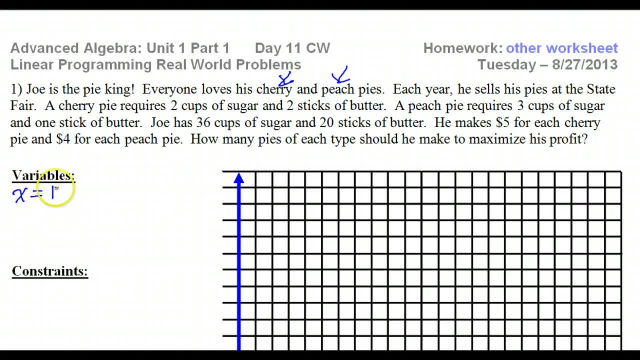 So the variables need to be: x will be the number of cherry pies and I'm going to let y be the number of peach pies. Now I'm looking for constructions, Constraints, limitations, blah, blah, blah. peach pie, this cherry pie, that. 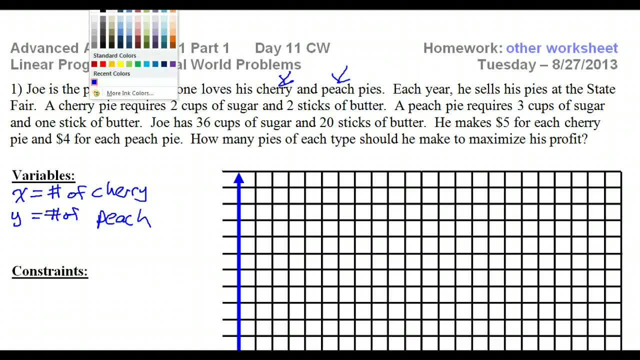 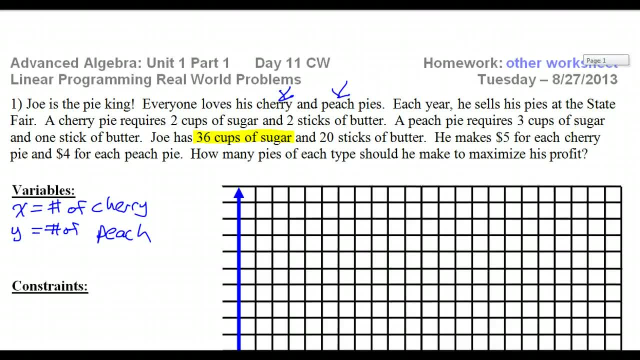 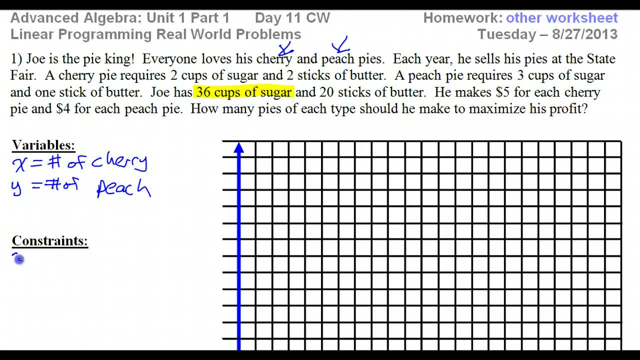 Joe has 36 cups of sugar. That's a constraint. 36 cups of sugar, that's all he's got. So that means there's a sugar constraint. So I'm going to write that down. I'm going to say: hey look everybody, sugar constraint. 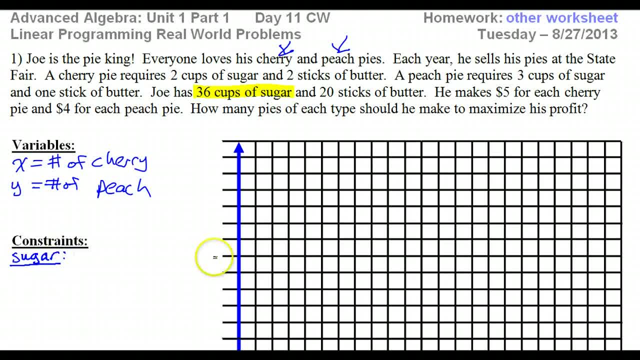 All right, now I'm going to write that sugar constraint. In fact, I'm going to squeeze it in right here. 36 cups of sugar, that means whatever else happens, it's got to be less than or equal to 36.. 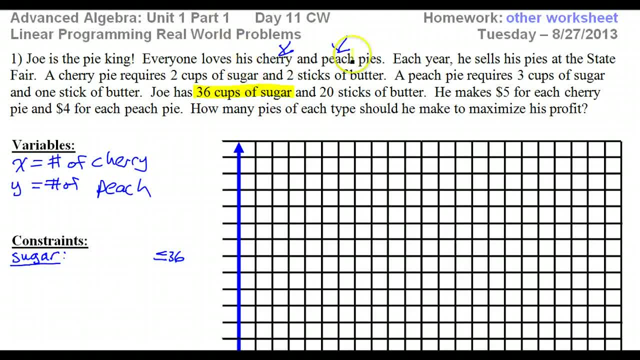 So now I'm going to scan the problem, looking for everywhere they mention sugar. All right, each year he says a cherry pie requires two cups of sugar, blah, blah, blah. Peach pie requires three cups of sugar. Okay, The other two things that go with sugar. 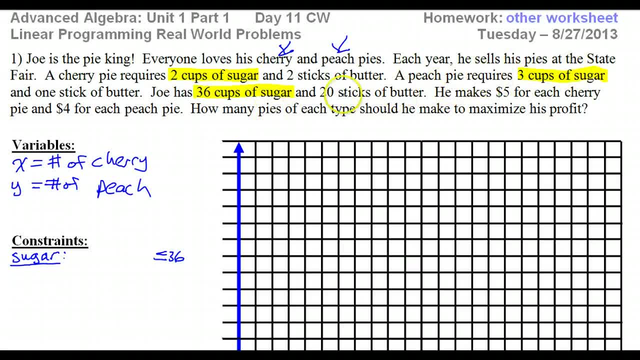 So the cherry pie was x, peach is y, so that's going to be 2x plus 3y. So the sugar constraint is 2x plus 3y, is less than or equal to 36.. Now I'm going to look for another constraint. 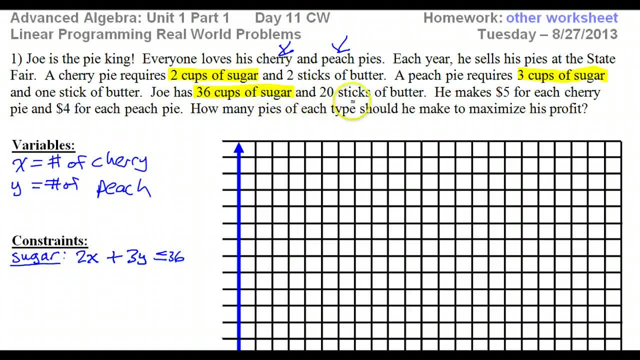 It's probably near the first one. He has 36 cups of sugar and 20 sticks of butter. Guess what? 20 sticks of butter? That's another constraint. Okay, 20 sticks of butter. So now I'm going to look through the problem, for everywhere they mention butter. 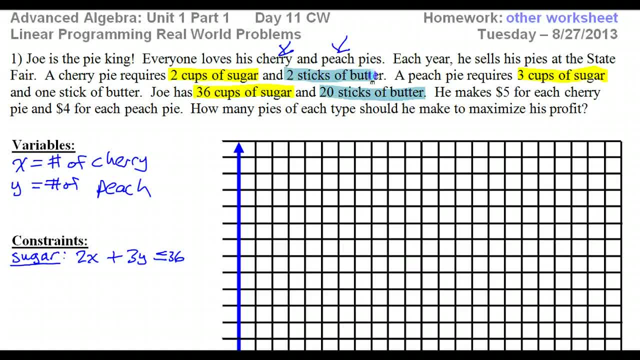 Blah, blah, blah. cherry pie: two sticks of butter. Peach pie: one stick of butter. All right, so look at this. Two sticks of butter, one stick of butter total 20 sticks of butter. Okay, Okay, let me use red this time. 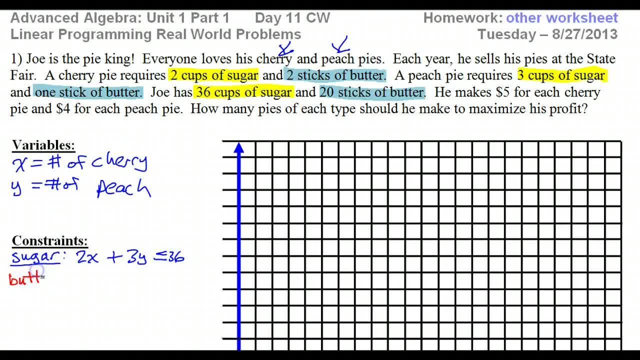 So this is a butter constraint. Okay, So two sticks of butter. So this is going to be: 2x plus y is less than, or equal to 20.. So 2x plus y is less than, or equal to 20.. And then there will always be the reality constraint. 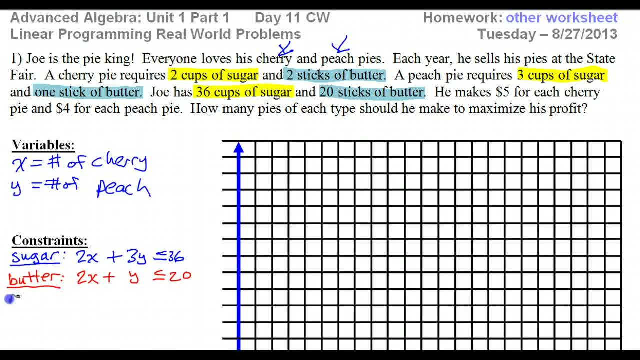 So we're going to look at the reality constraints for a problem like this. Okay, reality and the reality constraints are: it can't have negative pies, so x has to be greater than or equal to zero and y has to be greater than or equal to zero. 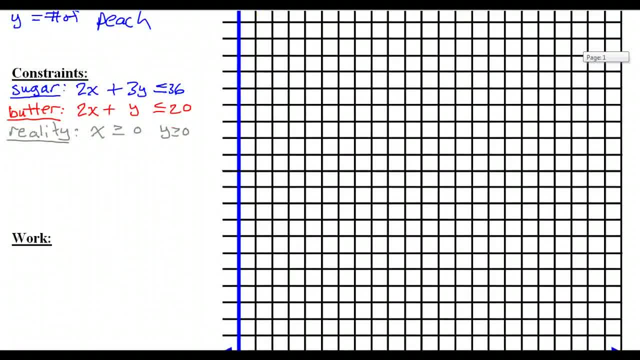 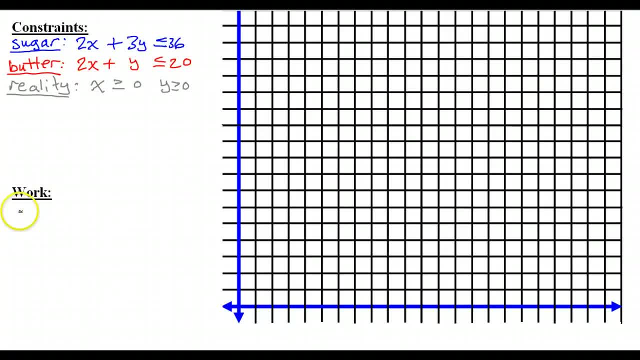 So those are our three constraints. Now we need to work them and graph them. So, looking at the blue one: Okay, Okay, You know, I've got that. 2x plus 3y is less than or equal to 36.. 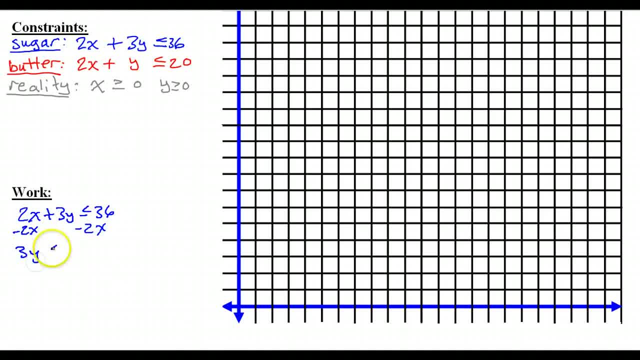 I could subtract 2x from both sides, So that gives me: 3y is less than or equal to negative 2x plus 36.. I need to divide by 3 everywhere, so that's going to look like this. So that's going to give me: y is less than or equal. 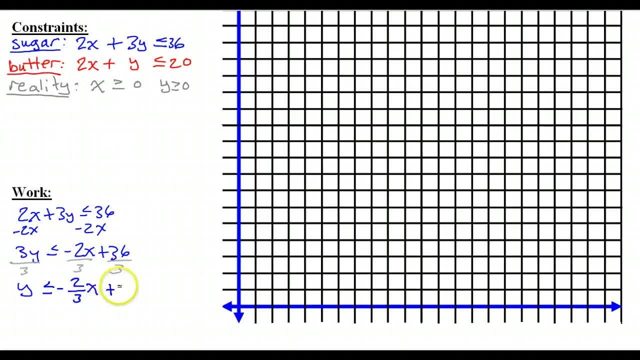 to negative: 2 thirds x plus 12.. Okay, so this is one constraint and I'm going to go ahead and graph it All right: 12, that's looking like a small enough number that should fit. So 1,, 2,, 3,, 4,, 5,, 6,, 7,, 8,, 9,, 10,, 11,, 12, down 2 over 3.. 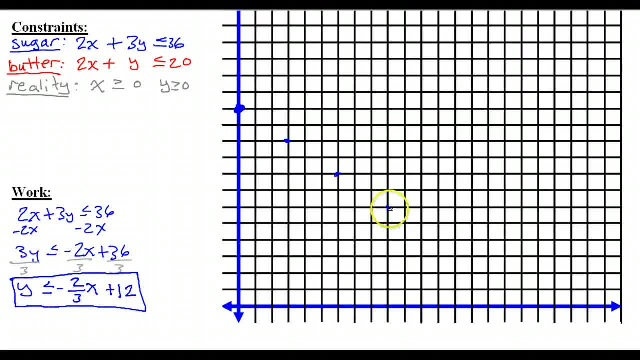 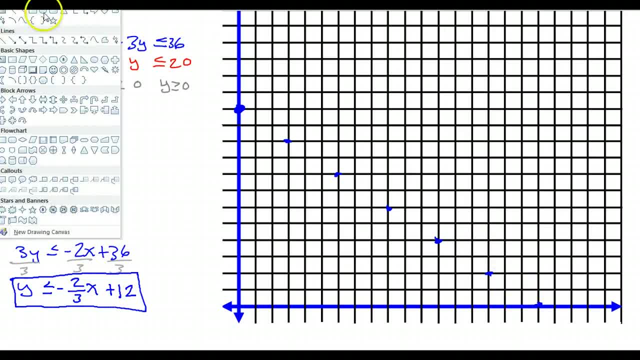 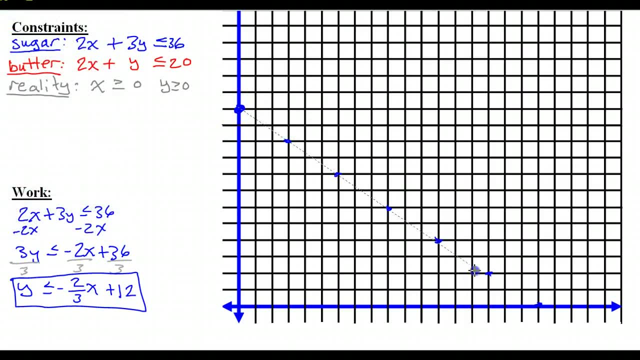 So down 2 over 3.. I'm working it, I'm doing it, I'm living it, I'm loving it. Okay, so that's going to look. whoops, I missed. I hate it when I miss, So that's going to be like this: 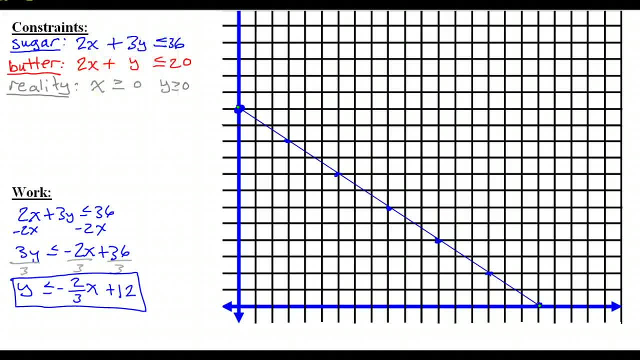 Let's make it blue and let's make it a little bit bigger. This is less than or equal to, so I'm going to put the grass that little bit over here. A little bit of shading on the below side of this line. 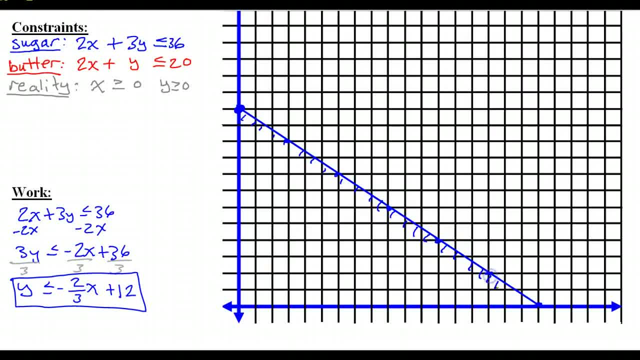 Just enough to remind me to stay on this side of the line As long as I'm here. I might as well shade in the reality constraints as well. All right, the reality means we stay on this side of the line, of course. 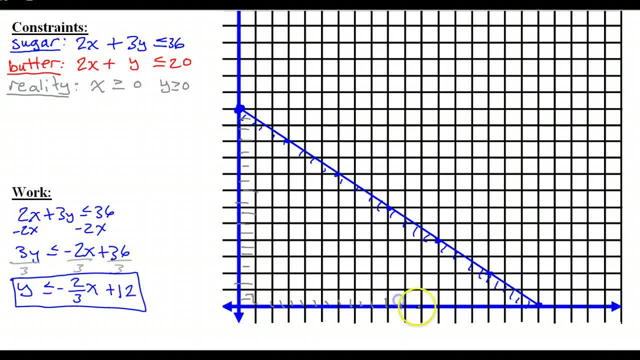 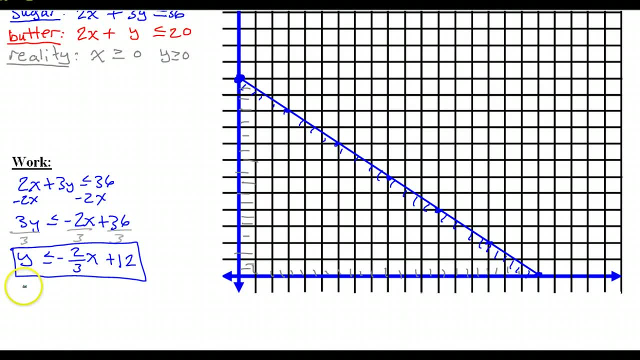 and we stay on this side of the line. Okay, this grass represents This grass represents my reality. constraint, Now the butter constraint. Let's do that butter constraint. Let's do it in red, So that constraint went: 2x plus y is less than or equal to 20.. 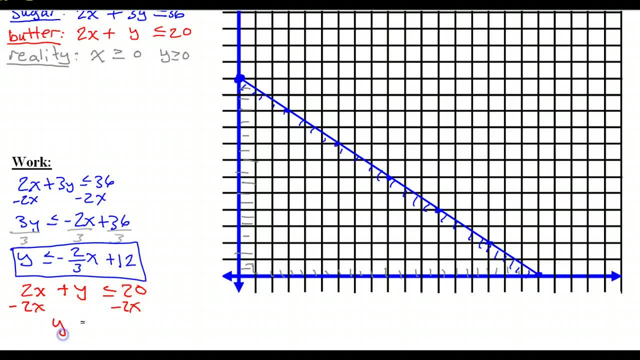 Subtract 2x from both sides, That gives us y is less than or equal to negative 2x plus 20.. All right, 20 is kind of a big number, but this goes up to like 23,. so I'm still over here. 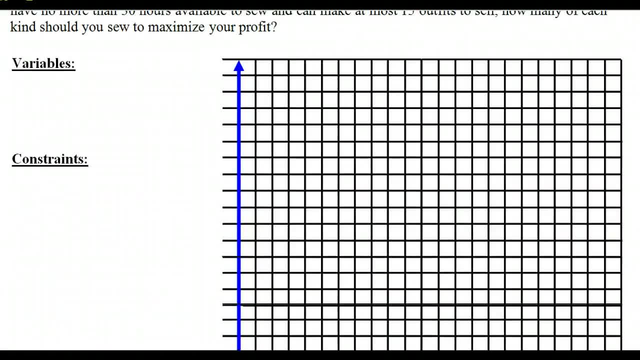 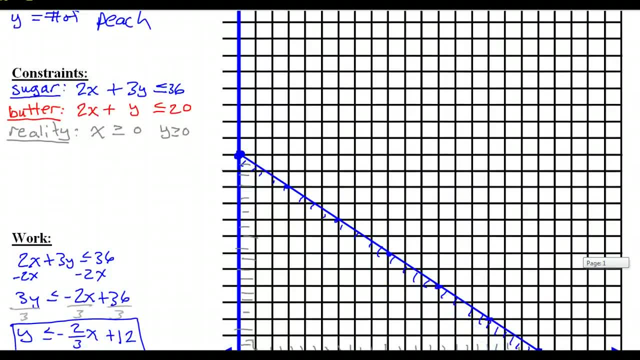 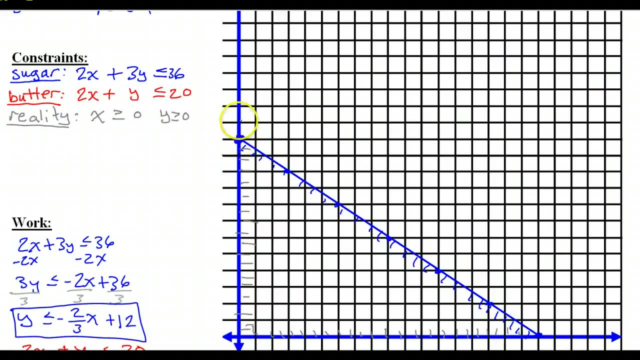 So I'm still okay. Okay, well, where did I go? Where did everything go? Scary. Okay, so this one is at 12.. So 13,, 14,, 15,, 16,, 17,, 18,, 19.. 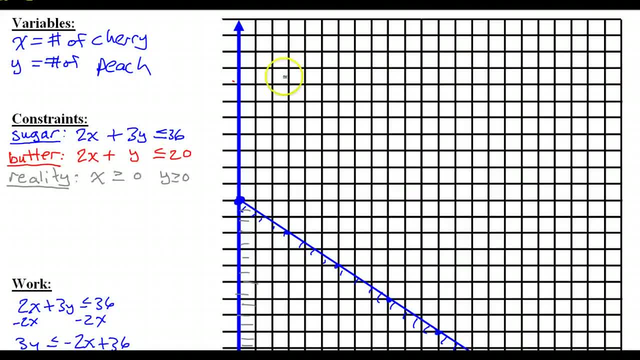 So close. All right, that's 19.. I had to mark it, So that's 20.. So then the slope is negative 2.. So I'm going to go down to over 1 like this. Okay, Okay, Okay. 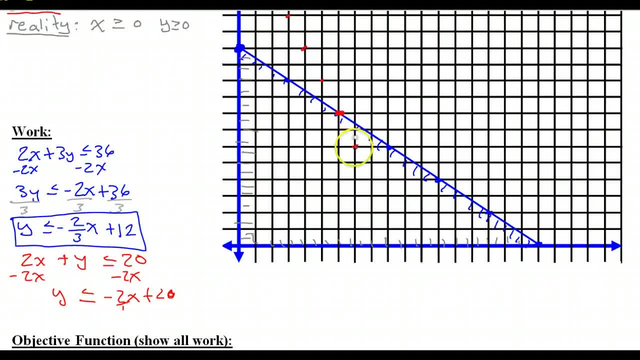 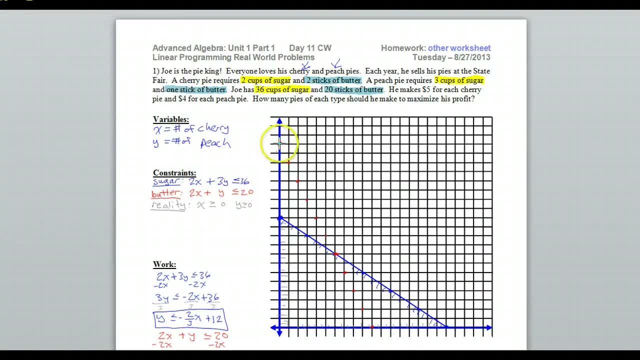 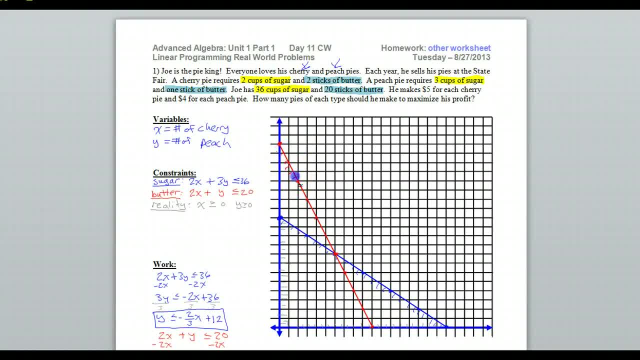 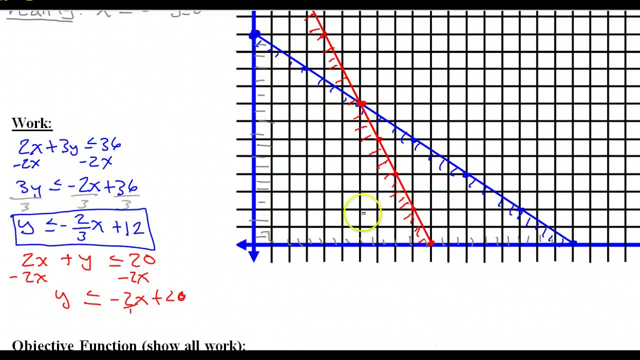 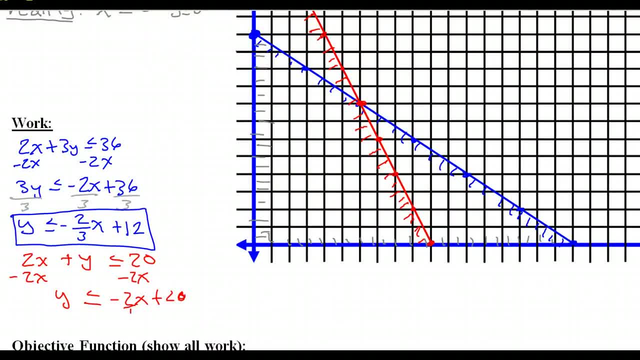 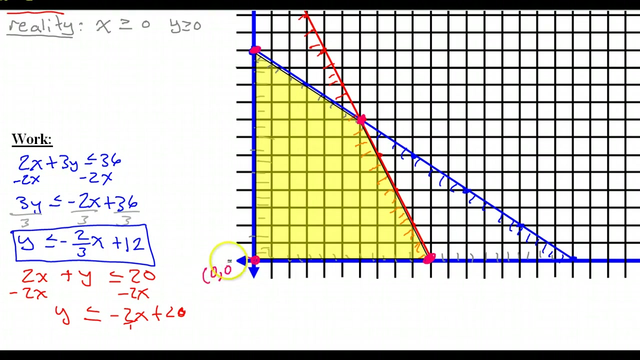 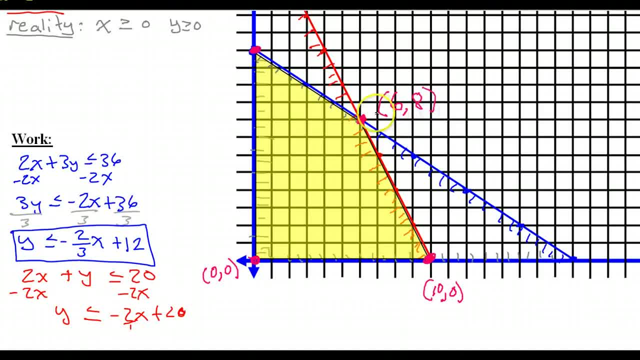 So this is 6, 8.. And this I think was 12, right: 2, 4,, 6, 8,, 10, 12.. All right, so this one was 0, 12.. 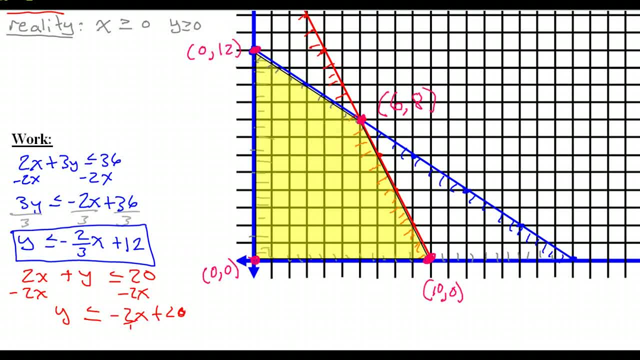 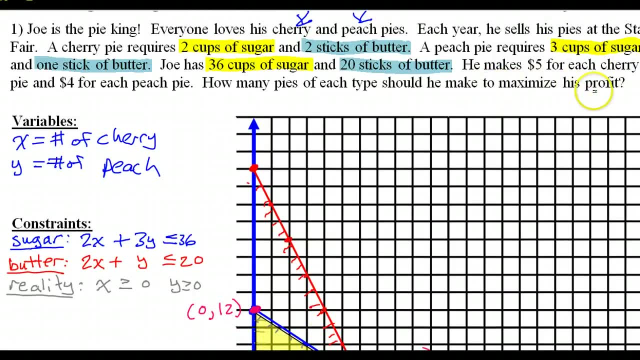 So those are the four vertices. Now we need to substitute those into our objective function. but so far we haven't written the objective function, so we need to do that, All right. so what is our objective? To maximize profit. So we need a profit equation. So the profit equation is going to run like this: 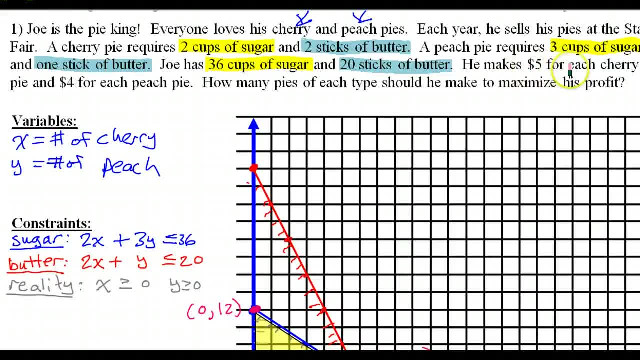 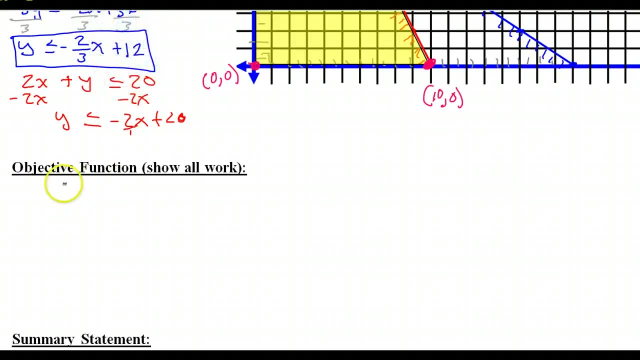 Okay, he makes $5 for each cherry, $4 for each peach. All right, that's pure profit. So that's 5x plus 4y. So when we make our profit equation it'll look like this: Profit: 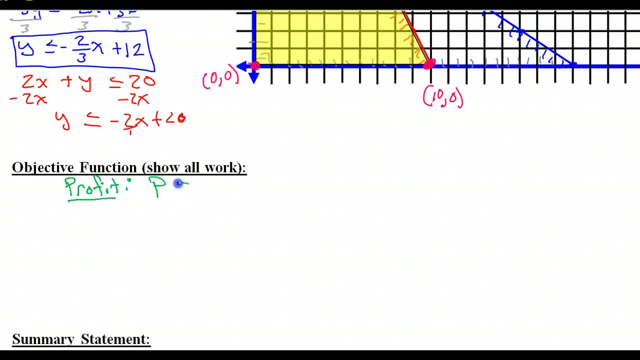 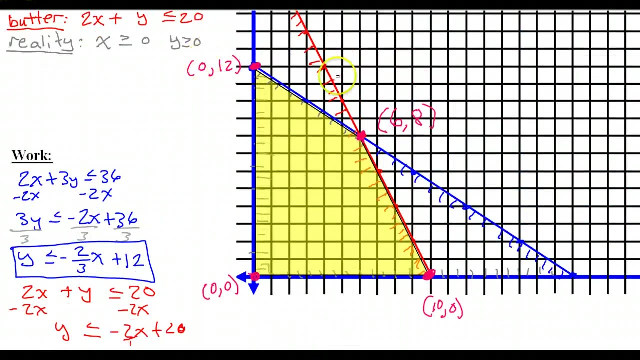 5x plus 4y. So we will just take our four points, one at a time, substitute it in. So if I put in 0, I get 0. I'm going around the clock clockwise. So next, 0, 12.. 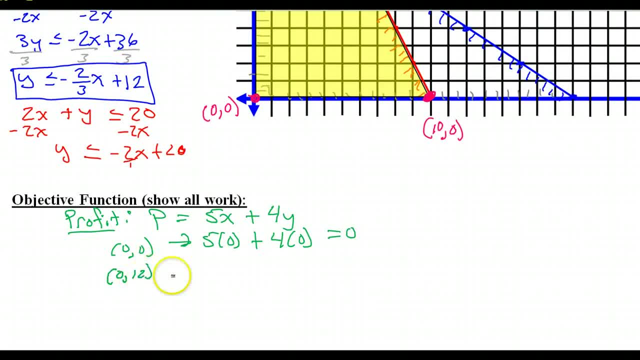 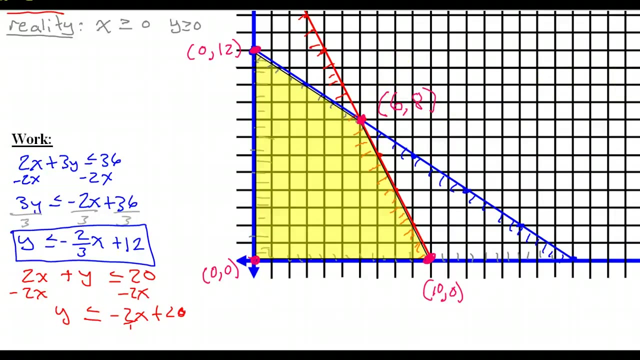 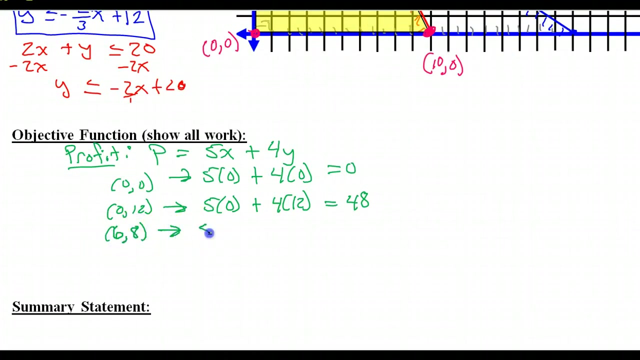 If I put that in All right, Obviously that's nothing, so that's 48. All right. next I have 6, 8. I'm doing this one: 5, 8. 9. 20. 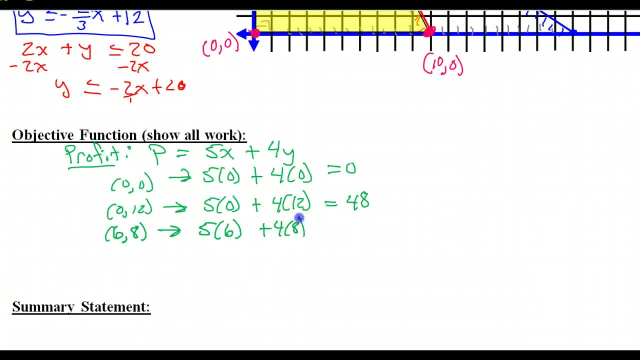 That's 62.. And finally we have 10 comma 0. So that's 5 comma 10, I mean 5 times 10 plus 4 times 0. So that's 50.. OK, so our max is right here. 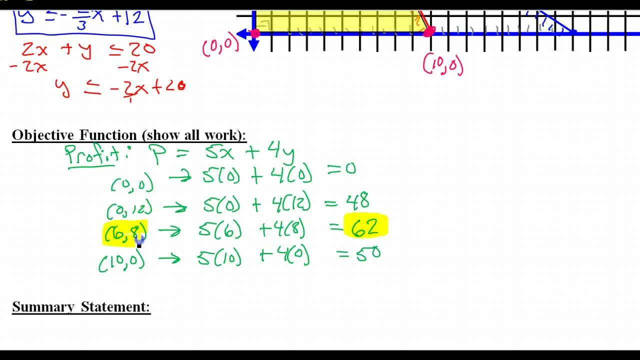 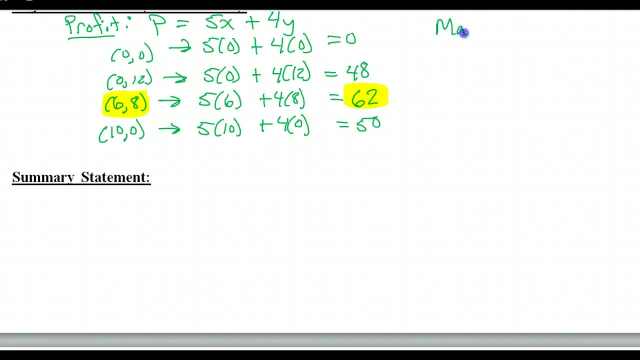 Max of 62 at that point, right there, And let's just write that down before we move on. So we have a max of 62 at 6 comma 8.. And for the record, we had a min of 0 at 0 comma 0.. 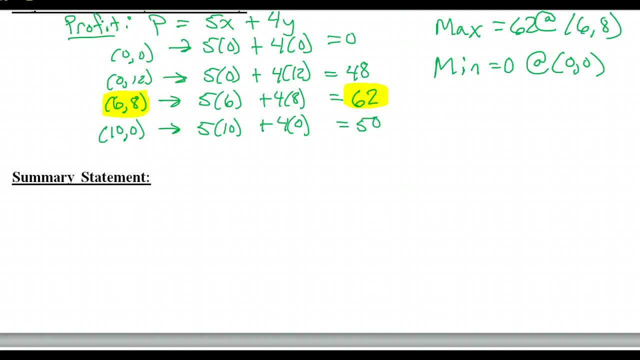 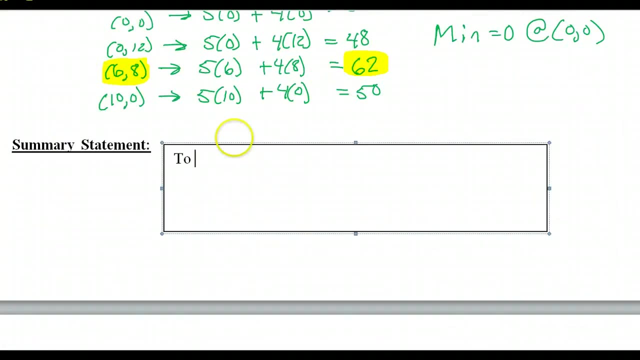 So summary statement. Hey, where's my text box? All right, this is a person, Joe. Joe is the pie king. OK, notice that I'm going to mention all three of these numbers: the 62,, the 6, and the 8.. 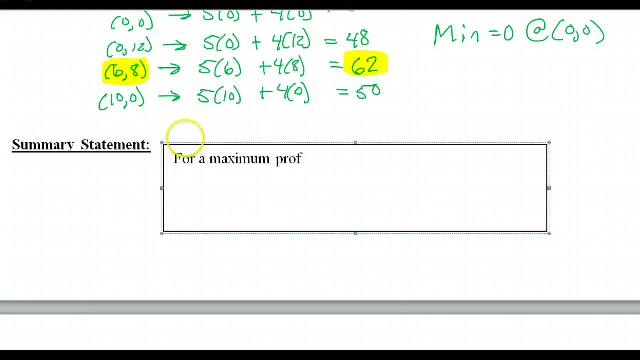 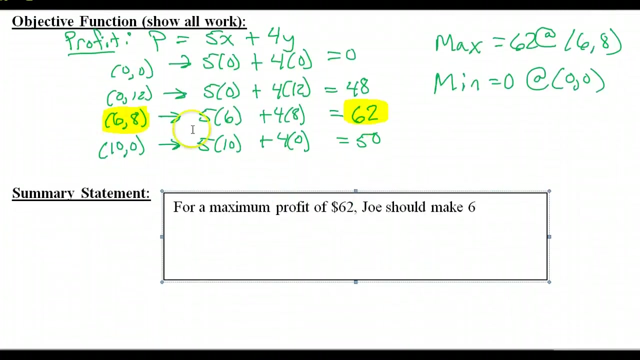 For maximum profit of $62,, Joe should make 6.. Now let me just make sure about the variables. All right, cherry pies and then peach pies. OK, so cherry peach. So 6 cherry pies And 8 peach pies. 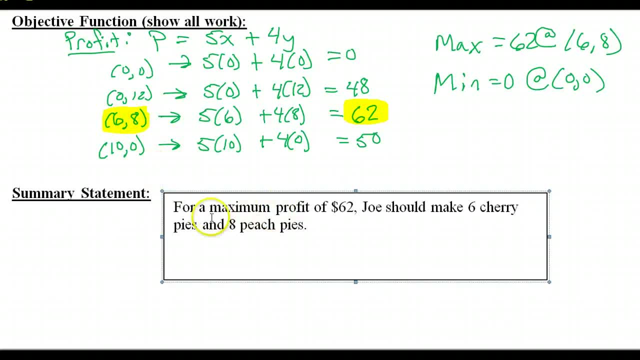 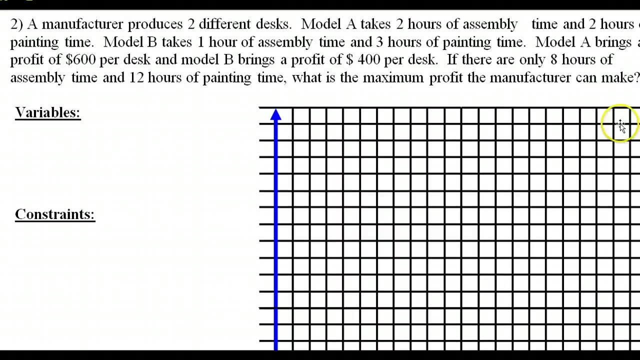 OK, 6 and 8.. Boom Done. All right, that is how you do that, my friends. OK, that was number 1.. Let's look at number 2.. All right, desks. Two different kinds of desks. 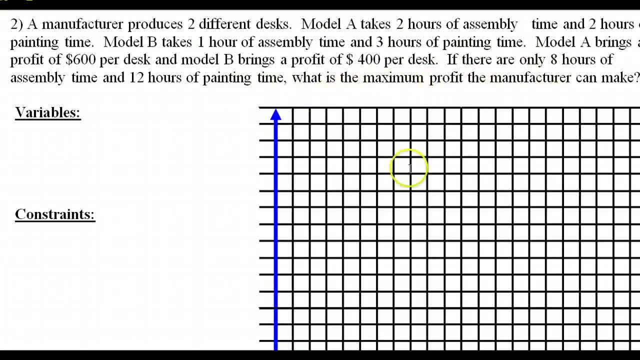 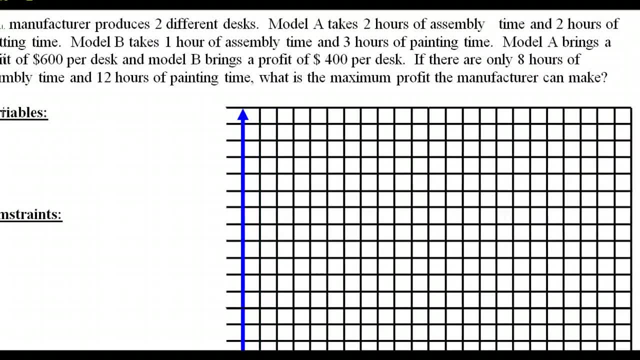 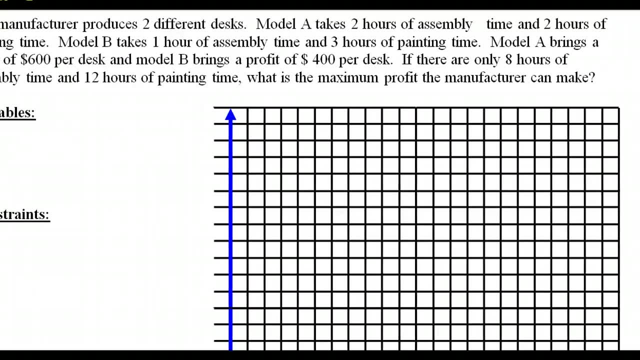 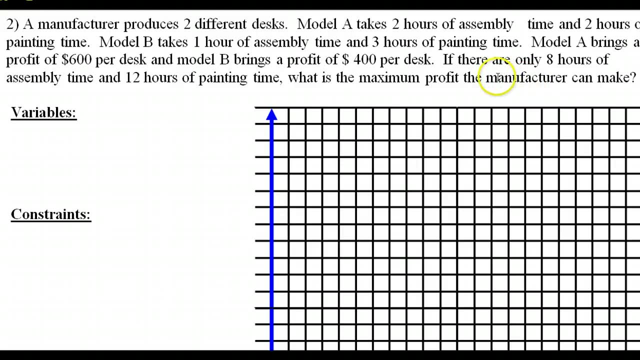 Blah, blah, blah. what's the maximum profit he can make? OK, hold on. Hmm, OK, So saying what's the maximum profit you can make, That's something we always answer anyway. But OK, he's got the total. 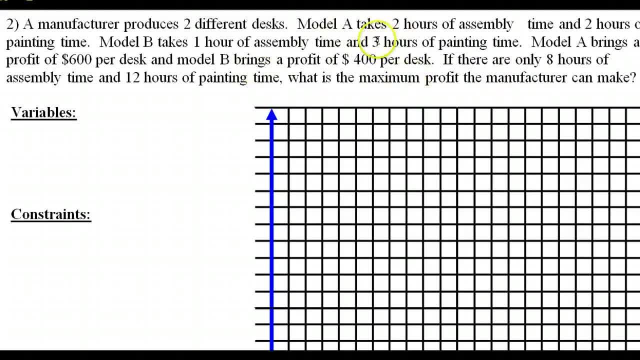 OK, All right, OK, $62. $62. $63. $64. $64. $64. $64.. two kinds of deaths. so we're we're gonna have to figure out how many of each kind of deaths he can make. it doesn't actually, you know, I was looking for it. 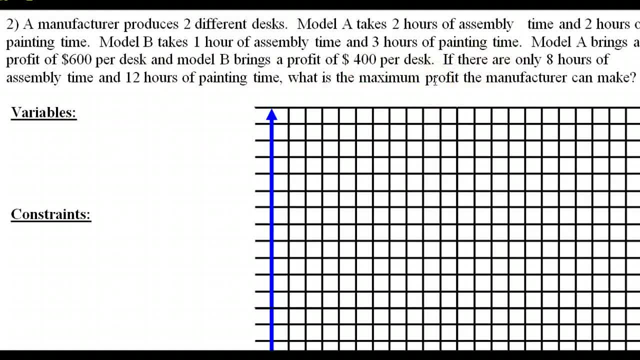 here at the end, like it normally will say, but this time it didn't actually say how many of each type of desk, it just went straight to the profit question. so, but we still have to know that the variables will be the number of each type of desk, so this one's a little tricky in terms of defining your. 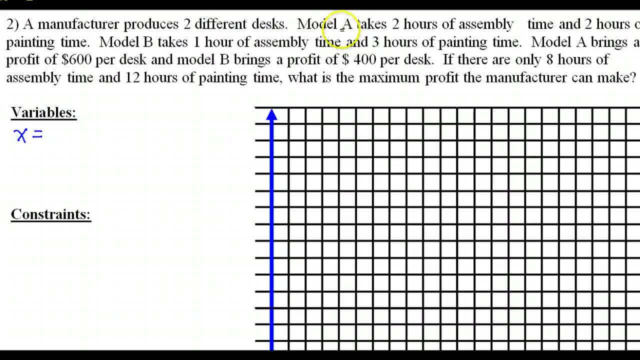 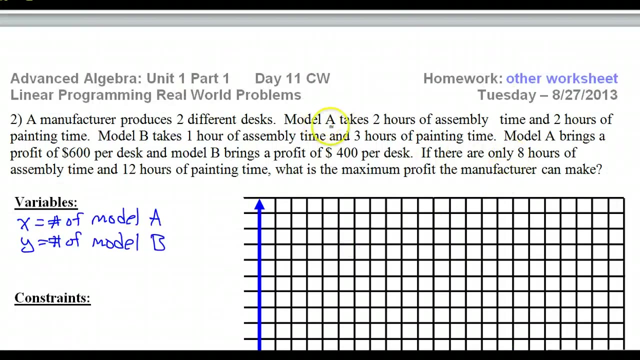 variables. all right, so two different kinds. so we have model a and model B. so I'm gonna let X equal the number of model models a and I'm gonna let Y be the number of models B. so time for the constraints me back, get out just a little bit. so let's see, model a brings a profit of this there. 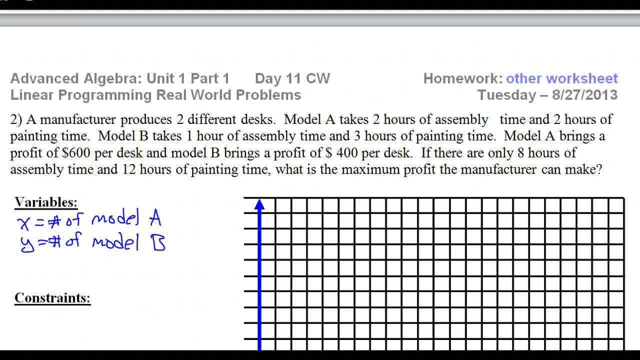 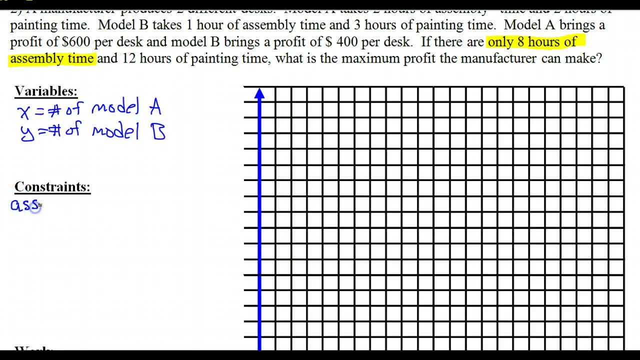 are only eight hours of assembly time. that's a constraint. only eight hours of assembly time, that tells me I'm gonna have an assembly constraint. so let me go ahead and write that down right now. assembly- okay, maybe I can just squeeze it in right here. only eight hours, that means. 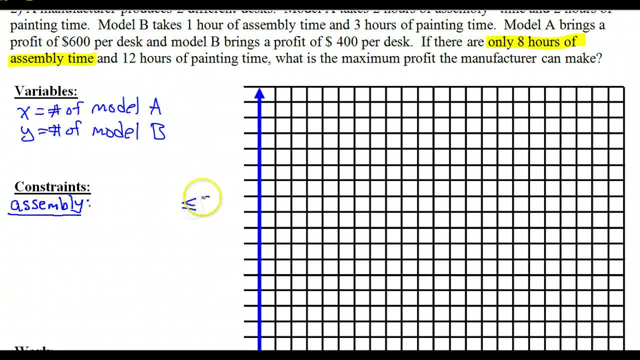 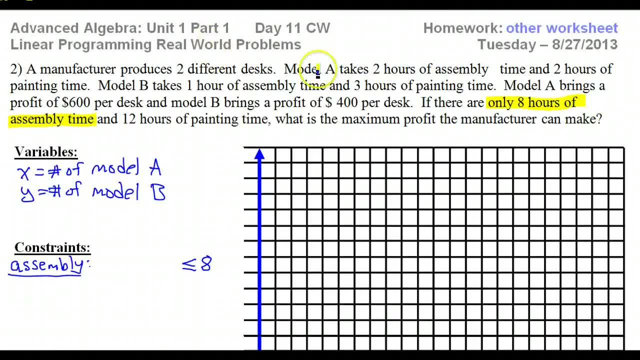 whatever else happens, it's going to be less than or equal to eight. so since we're talking assembly, I'm gonna scan through the problem and looking for every mention of assembly. model a takes two hours of assembly- blah, blah, blah. model B takes one hour of assembly. that's the rest of my inequality. 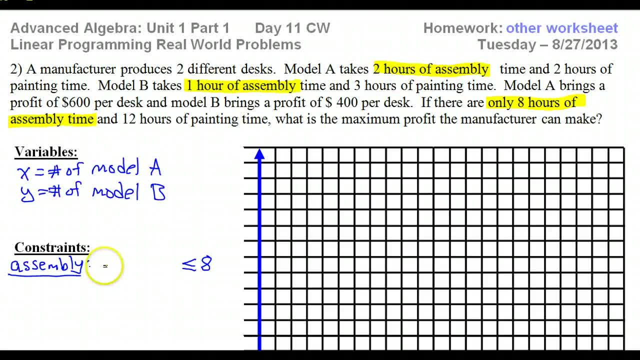 so that's going to be 2x plus y. so 2x plus y is less than or equal to 8. let's look for another constraint: 12 hours of painting time. there are only 12 hours of painting time. that's another constraint. all right, so I'm going to have a painting time constraint. put that one in red. 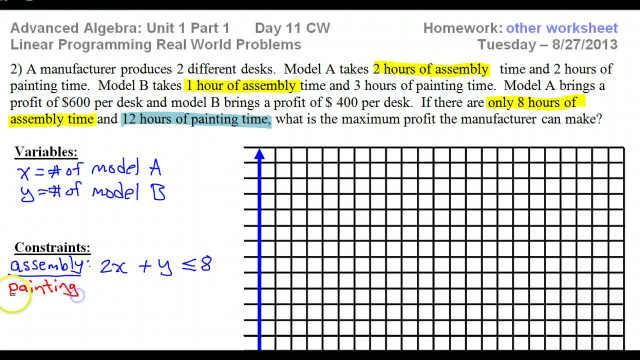 okay, all right, only 12 hours, so that means less than or equal to 12. so now I'm going to scan through the problem, looking for every mention of painting time. model a takes two hours of painting time- and I'll just leave it blue because we know that that's painting time- and model b takes three. 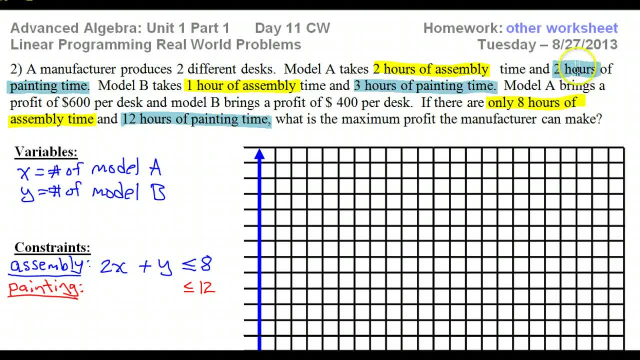 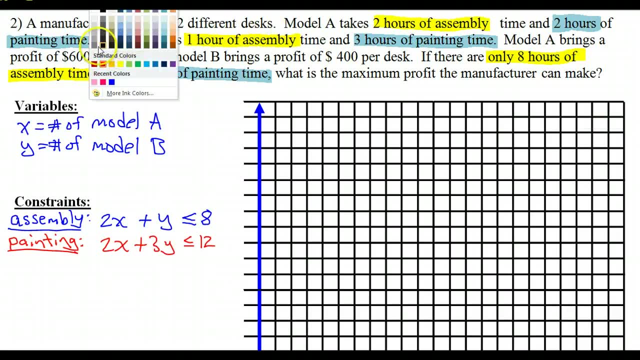 hours of painting time. So that's 2x plus 3y. So that's my painting constraint. Don't forget your reality constraint. We cannot have negative desks. So x has to be greater than or equal to 0, and y has to be greater than or equal to 0.. 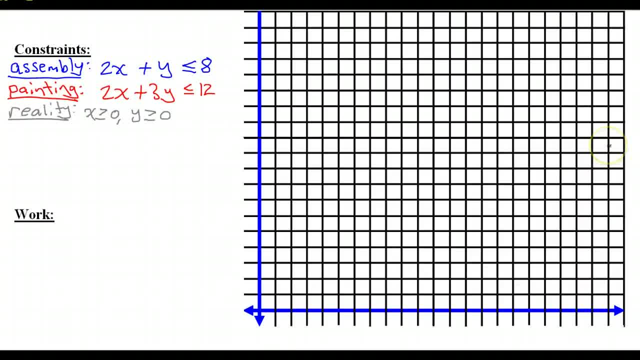 Let's work the constraints and graph them. Let's start with the assembly shown in blue. We have our 2x plus y is less than or equal to 8. subtracting 2x from both sides gives me y is less than or equal to negative 2x plus 8. I'm going to go. 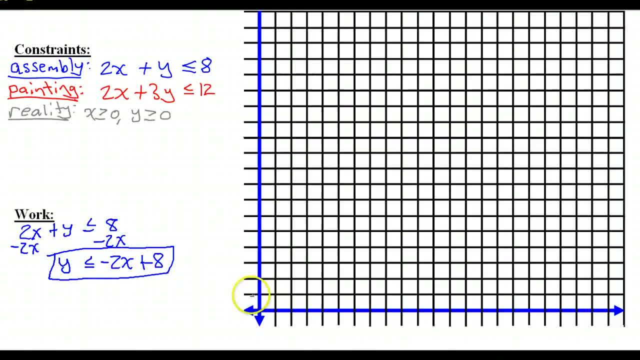 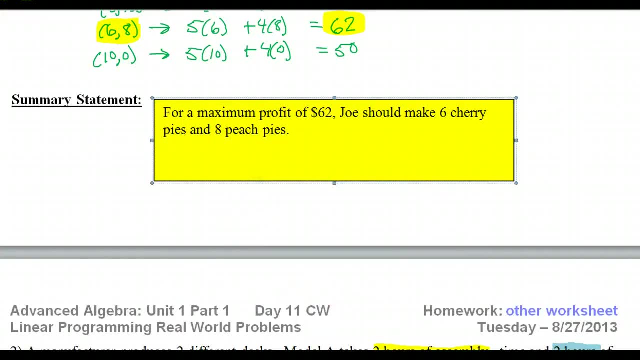 ahead and graph that. all right. so it's 1, 2, 3, 4, 5, 6, 7, 8. let's put a little 8 here to remind me- and this is down, two over one, like this: whoa, I wish it wouldn't do that. 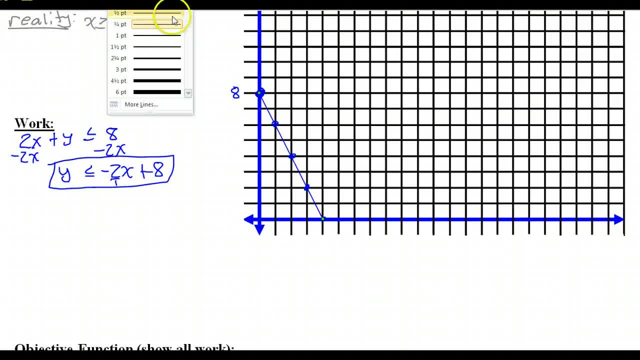 scares me. this is less than or equal to 2, so I'm going to put that little shading here here, Like grass growing upside down, Okay, and there's also the reality constraints, Which are like this. So so far, I have to be in this triangle, Whatever else happens. Let's look at the next constraint, the painting constraint. 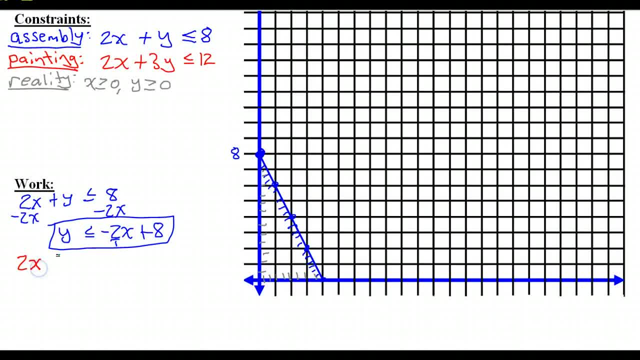 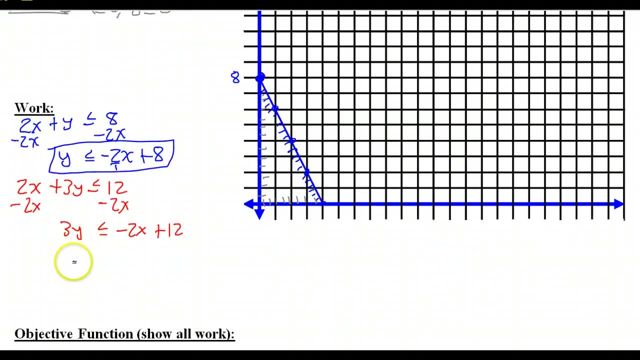 Which goes: 2x plus 3y is less than or equal to 12. If you subtract 2x from both sides, That's going to give me: 3y is less than or equal to negative 2x plus 12. If I divide everything by 3, 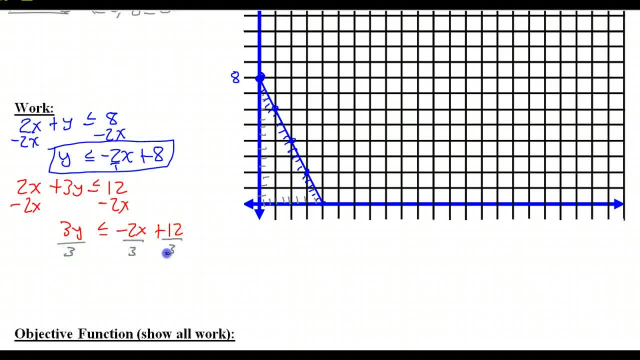 That's Going to give me y is less than or equal to negative 2 thirds x plus 4. so 1, 2, 3, 4, Right for my y intercept. and then down 2 over 3. so down 2 over 3, down 2 over 3. 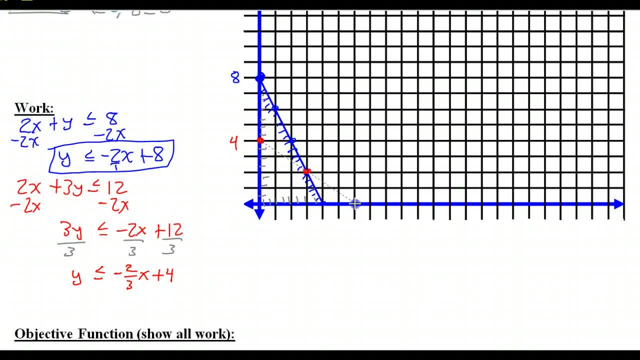 Estimated ح, lid2, 5xAH Less than or equal to Put the grass on the bottom side. I Don't even need to finish with the grass over here because I know I can't come out of the triangle So sometimes I skip it. So you can see that this little quadrilateral right here is going to be my shaded area. My feet are about this big profile, feeling right on the top of a tree right there. so when I guess what's the problem, I can scope out all this area. other are going to end up preserve all theobic evenly and that leaves all of the concrete in the other area. so I need to shape the tree as a beach in one class. as I唐u, I'll copy it before I make two East side sectors, should I, yes h, get a bay? on the other hand, 아마 I read off of a 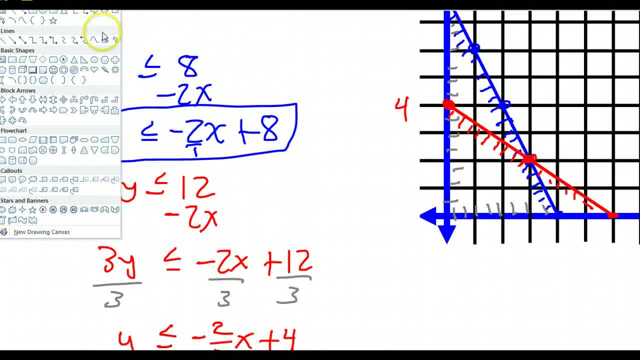 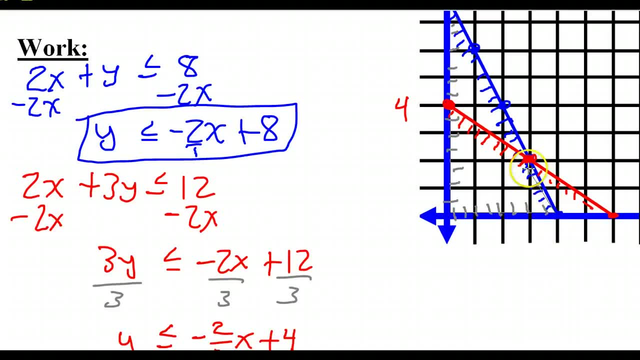 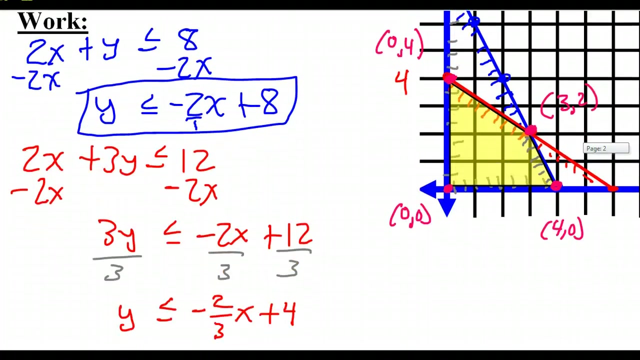 feasible region. Now we need those vertices which are here, here, here and here. So that is 0 comma 0,, 0 comma 4,, 3 comma 2, and 4 comma 0. So those vertices need to be put into our objective function. but we haven't created. 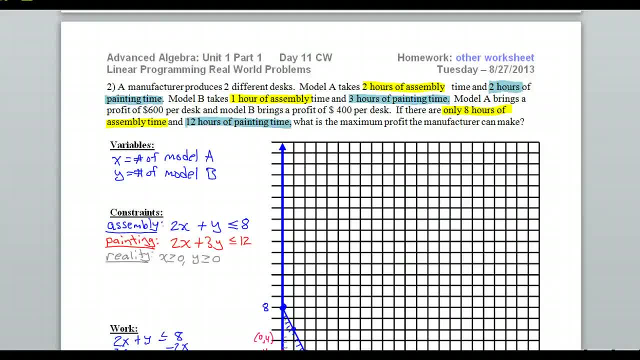 that yet, so we better go back and check it out. Our objective is profit, so we need a profit function. I'm going to do the profit in pink- Maximum profit okay. Model A brings a profit of $600 per desk. 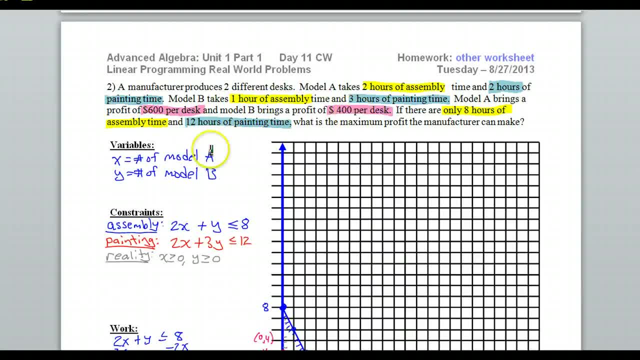 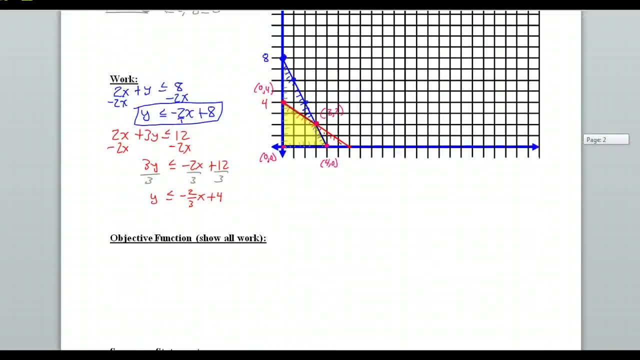 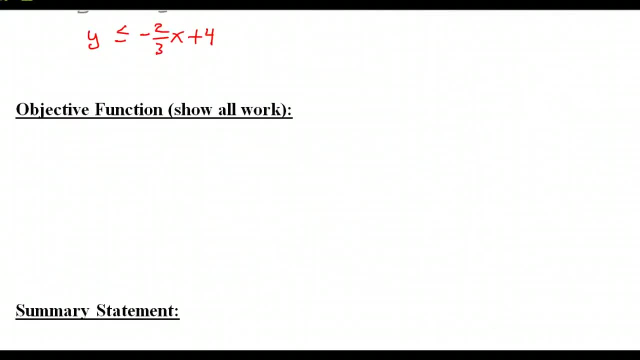 Model B: $400 per desk, So that's going to be $600.. $600 X plus $400 Y. So let's write that down, Okay, Profit P equals $600 X plus $400 Y, And into that function we will put. 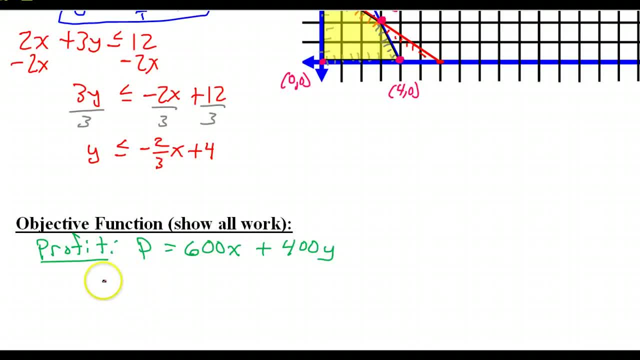 Just a reminder. the testing committee will meet in the PCR at 740.. Testing committee- PCR 740.. Thank you, Okay, 0, comma 0 goes in: Whoops 400.. Okay, That's going to give me 0.. 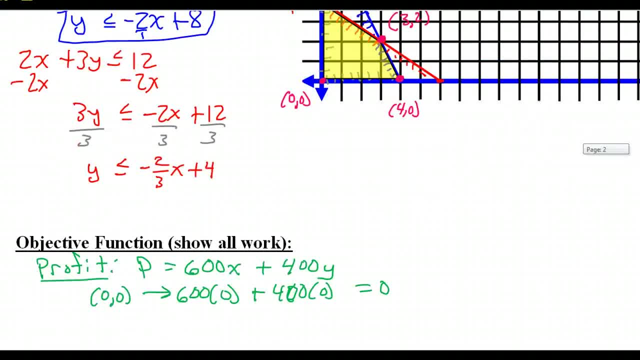 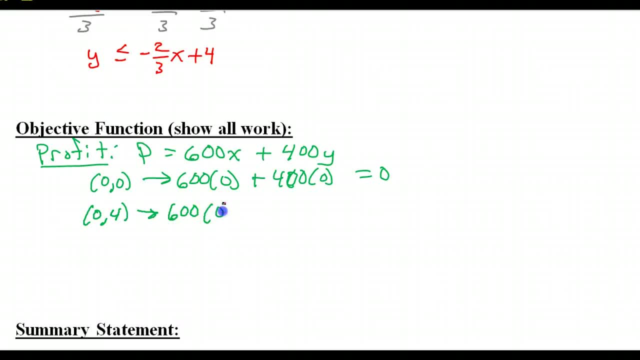 Next, I'm going to do 0 comma 4.. Okay, That's going to give me 0.. Next, I'm going to do 0 comma 4.. Okay, That's going to give me 0 because of the hundred. so and so. 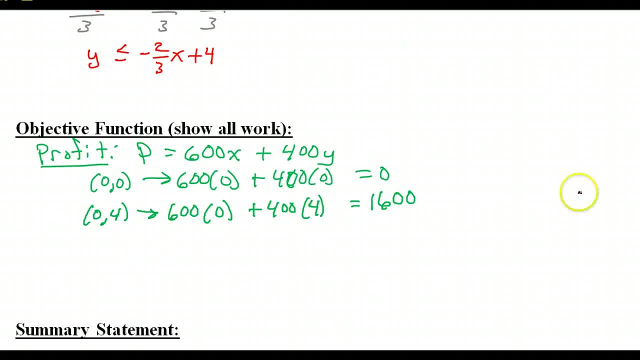 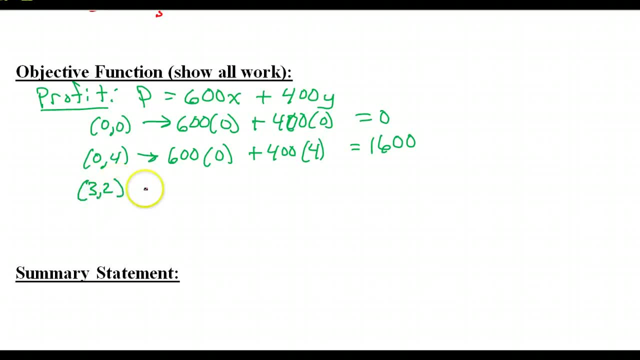 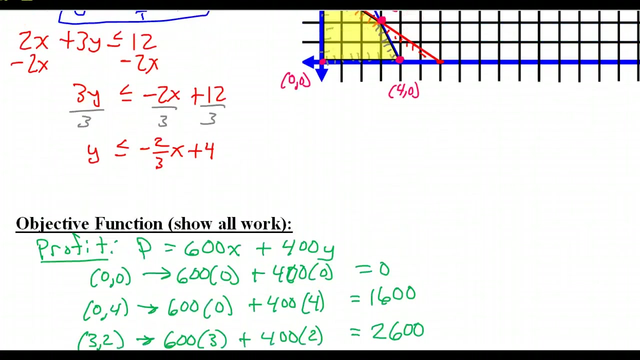 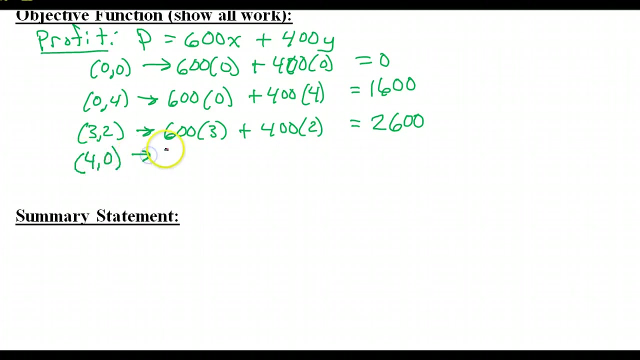 Okay, That's going to be 1600.. Next I'm going to do 0 comma 3.. Okay, That's 1.200.. Great is 2,600 and 4 comma 0. Whoops, So that's going to be. 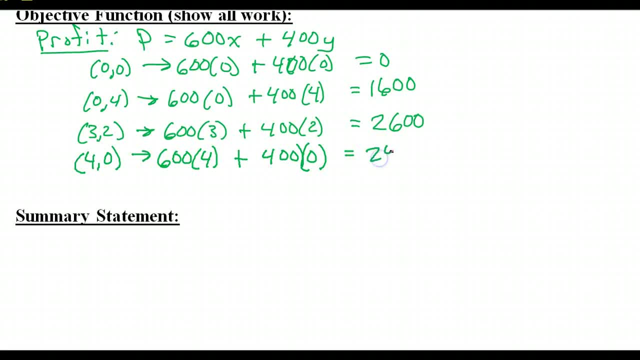 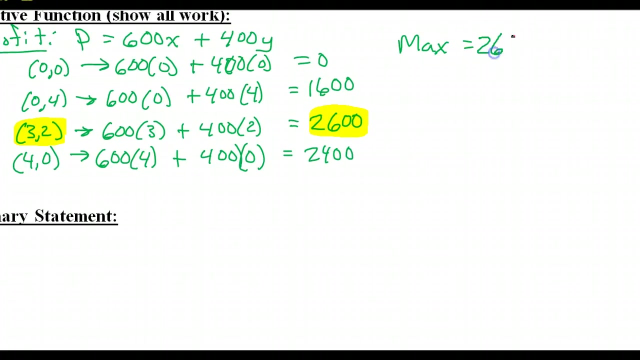 2,400.. So we have a winner. 2,600 is the max and it comes from this point right here. The maximum equals 2,600 at 3 comma 2.. This is not optional, by the way. Make sure you write this down.